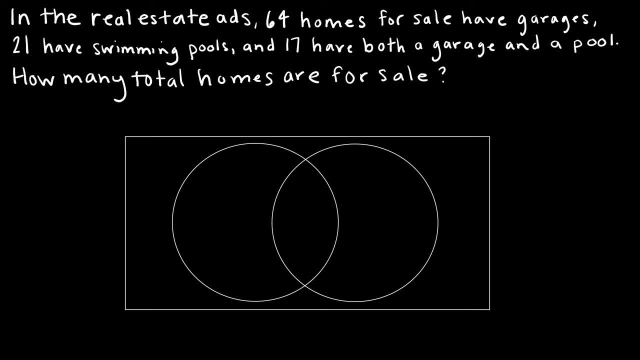 both How many total homes are for sale. Now, there's a lot of ways to go about this, but we're going to do it sort of the long way. We're not going to use our equation yet. So I know that in a Venn diagram, if this first circle represents garages and, say, my second circle represents pools, 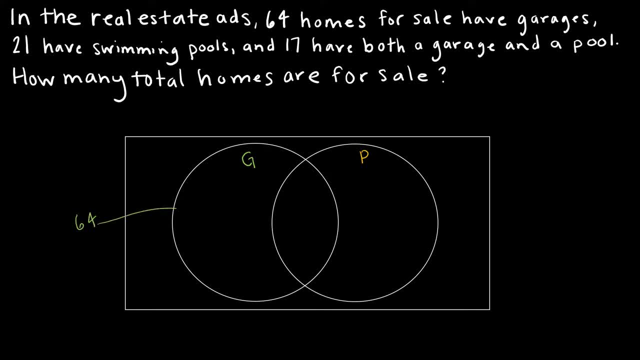 I cannot take 64 and put it right into this circle, because I know that 17 have both, And so I'm going to actually put 17 here in the middle, because 17 represents the intersection where there's both a garage and a pool. 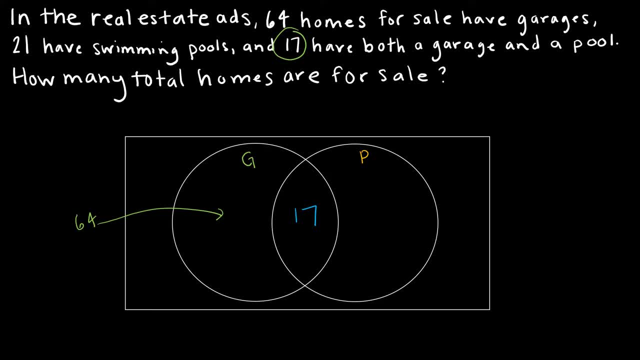 Which means The 64 has to be. everything inside this circle needs to be 64, and that includes the 17.. So I actually have to take 64 minus 17 to get 47, and that is the number that would go here. The other circle includes 21 total homes. 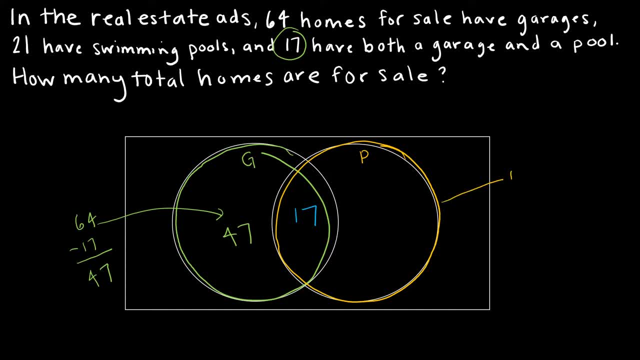 and that includes the 17 that I had before. So I had to do 21 minus 17 to get four. So there's actually only four homes here that have a pool but no garage. There are 47 homes that have a garage but no pool. 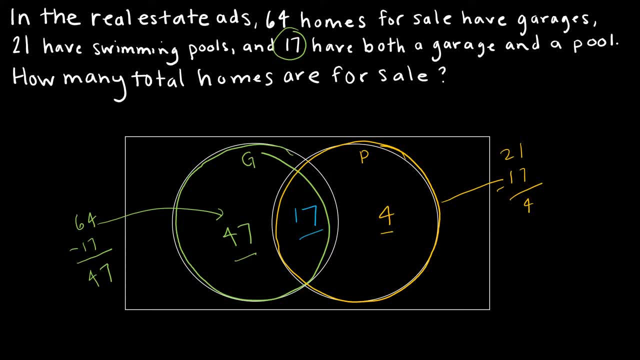 and then there's the 17 homes that have both. So how does that help me? Because now I can just add these values together. I can say 47 plus 17 plus four is the total number of homes for sale, which is, oops, 68 homes. 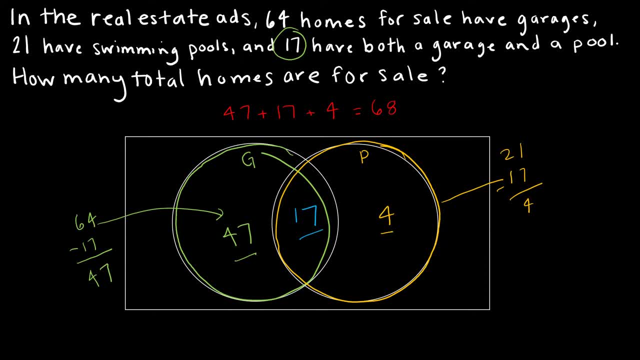 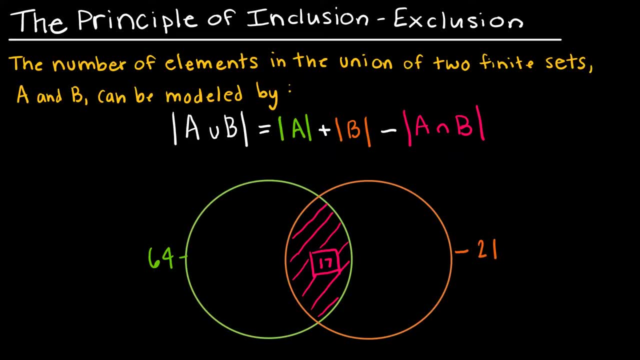 Now, of course, I don't want to have to draw a Venn diagram and do that math every single time, and so now let's look at the principle of inclusion-exclusion. So let's take a look at the principle of inclusion-exclusion, which is how we would do this. 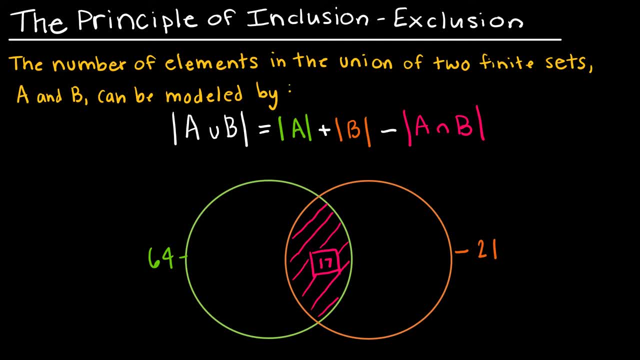 without having to draw a picture First, let's take a look at our previous formula. why? look at why it works. So the principle of inclusion-exclusion says, instead of doing it the way we did it before, where we have to sort of find each section of our Venn diagram, 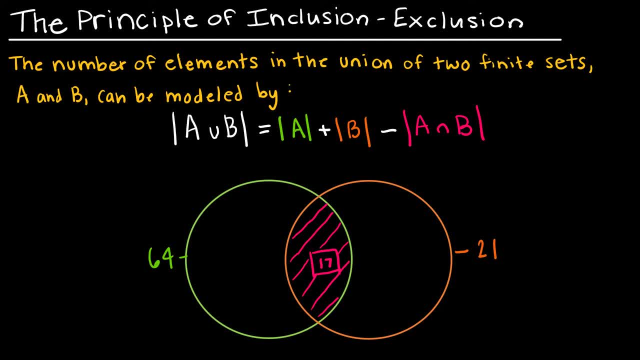 I can just take the cardinality, or the number of elements of set A plus the number of elements of set B minus the intersection, and that should give me all of the elements in the union. So we'll do it with our example that we just went through in just a moment. but let's take 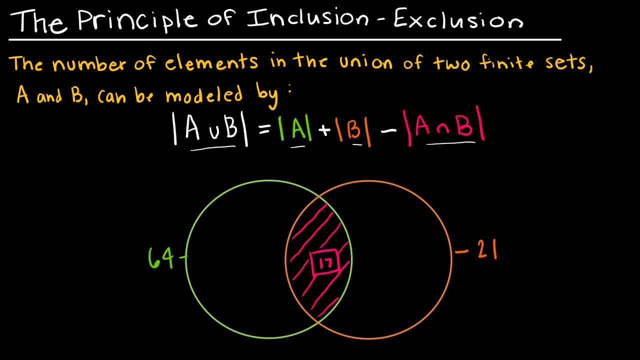 a look at why this works. When I look at set A, what's being added is everything in this section, as well as everything in this section. And when I take a look at set B, what's being added is everything in this section, as well as everything in this section, And so this section has been counted one time. 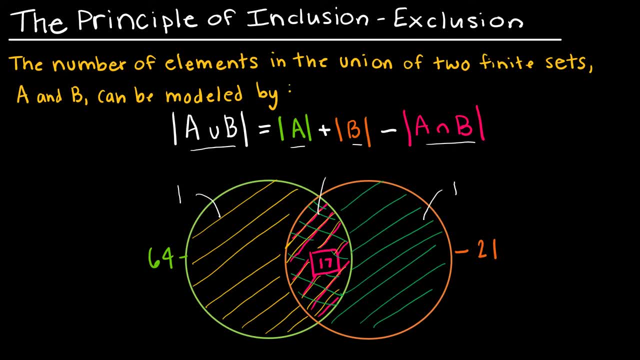 and this section has been counted one time. but this section got counted two times and that's not okay because we don't want it counted twice. So notice: what happens here is: I'm just subtracting the intersection of the intersection One time so that everything is being counted once. So this principle then says: I can take 64,. 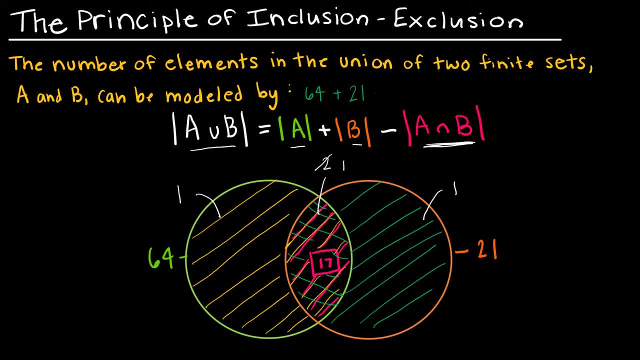 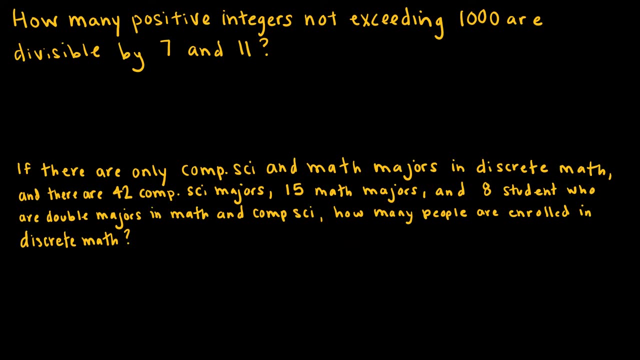 I can add 21, and I can subtract 17, and that will give me the same answer that I got using the other method, and that answer was 68.. So let's take a look at a couple of examples Using the principle of inclusion, exclusion. and again, this is just with two sets. 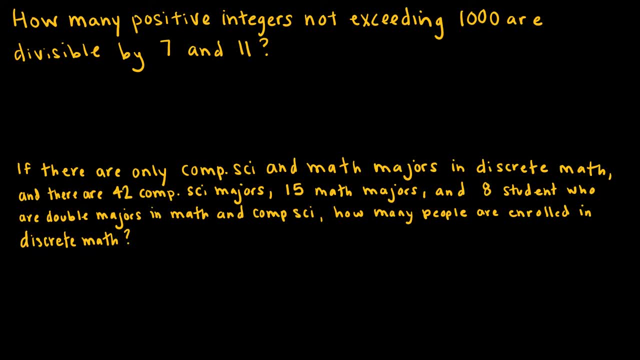 so we haven't looked at anything with three sets yet. This is how many positive integers not exceeding 1000, so 1000 is the top integer that I'll be looking at- are divisible by 7 and 11.. So I'm looking for the union of sets of divisible by 7, which we'll call A union divisible by 11,. 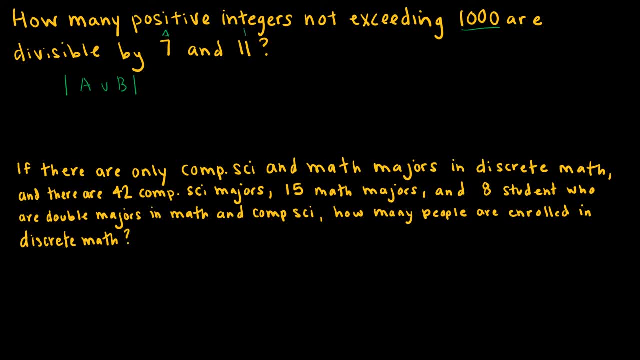 which we'll call B, And that means I need to find the number of items or elements in set A plus the number in set B and subtract the number. that are basically divisible by both 7 and 11.. So we're just going to use a good 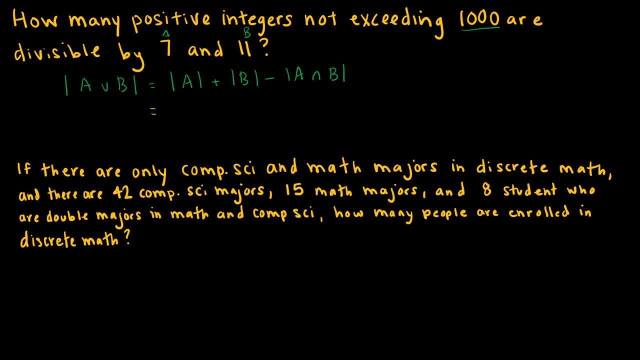 old floor function for this and we're going to say the number of elements in set A would be 7 and 11.. 1,000 divided by 7, except I want the floor function, because the floor function is just going to round it down. I'm going to add to that the number divisible by 11,. 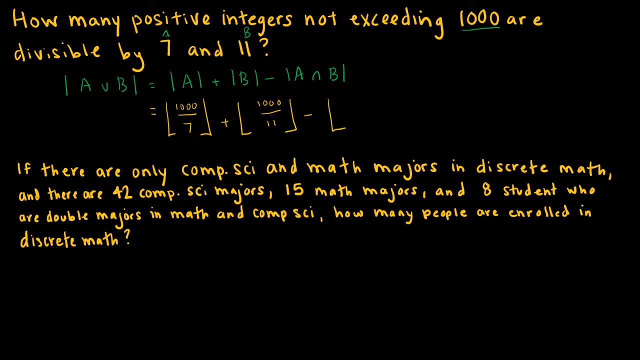 and then I'm going to subtract the number divisible by both 7 and 11, which would be 77, 7 times 11, so I'm going to divide by 77, and that's going to give me my final answer. 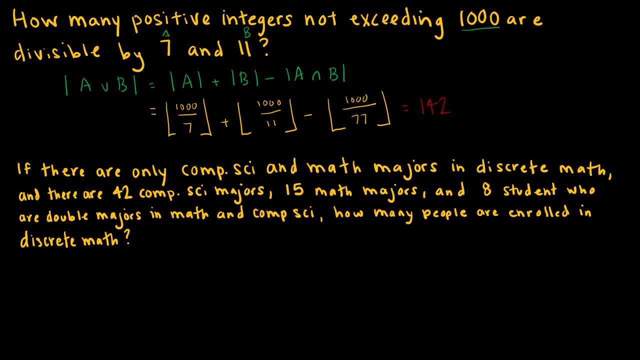 So turns out, there's 142 that are divisible by 7,, there are 90 divisible by 11, and there are 12 that were counted twice, once in A and once in B. so I have to take it away once and I get to 20.. 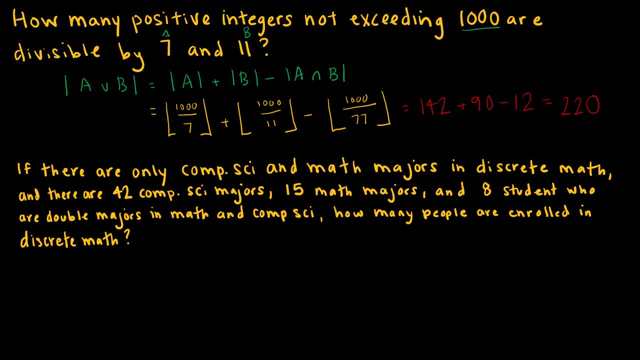 Second example: same problem, Same idea. I'm looking at computer science and math majors. so if I want the number of math majors union, the number of computer science majors, because that would be the total number of people in discrete math, then I would take the number of math majors: 15,. 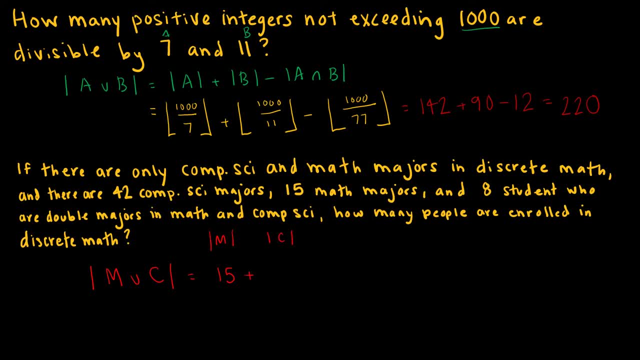 plus the number of computer science majors, which is 42. And I'm going to subtract the total number of math majors, which is 15,, And I would subtract anyone that was in both category, both math and computer science, which looks to be 8.. 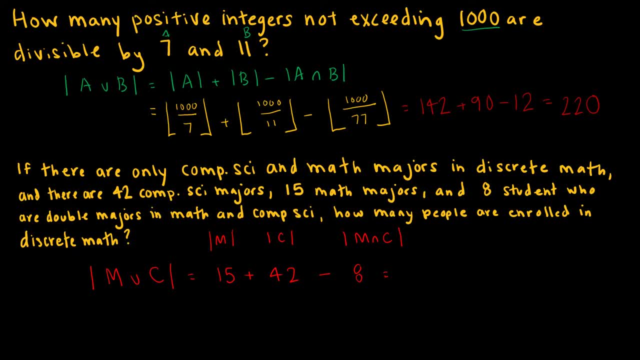 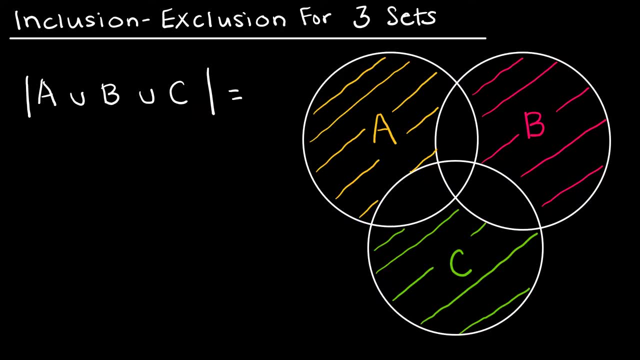 So I'm going to add 15 and 42 and I'm going to subtract 8 and I end up with 49 as my solution. So now let's look at inclusion exclusion for three sets, so we can start to come up with possibly a pattern. 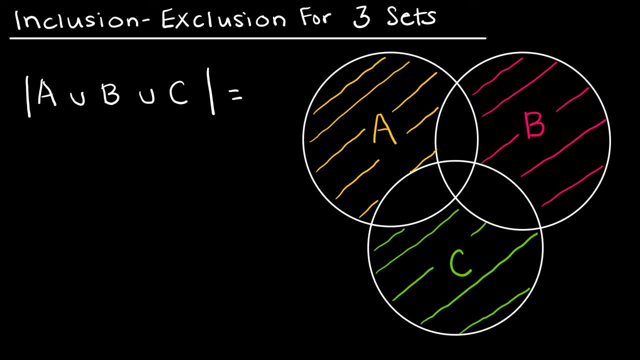 I want to add A, B and C. I want to find the union of those three sets. So I'm just going to sort of use a counting mechanism here and I'm going to start by adding A and B and C And let's see where we stand when I do that. 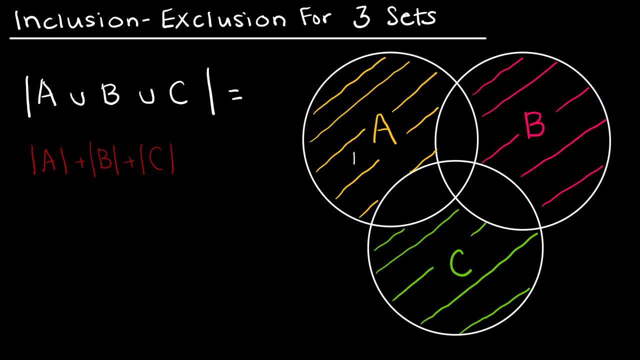 This section has been counted one time. This section is being counted once. This section is being counted once. This section is being counted once. That's just for A For B. I've got this section being counted once and then this section. 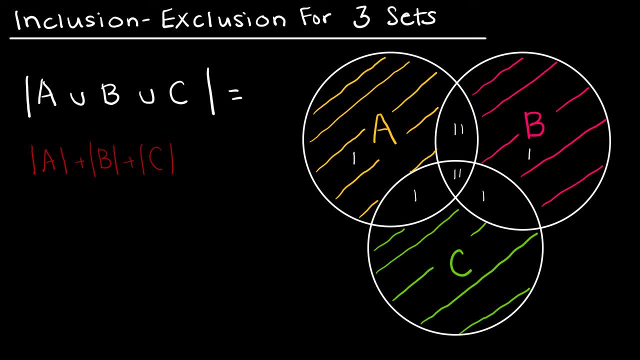 this section and this section And then, if I look at C, I've got this section being counted once and then I've got this section and this section and this section. So what it looks like is I've got a problem Because A, B and C- the parts that I colored in with the pretty colors- are all counted once. but I want to count everything once and I've got some issues because there's some things being counted more than once. 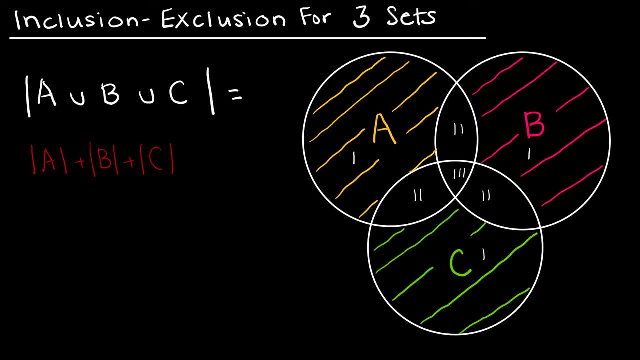 So now let's go about subtraction. So if I wanted to subtract, what if I subtracted A intersect B and A intersect C and B intersect C? So if I subtract all of that, let's see what's being counted now. 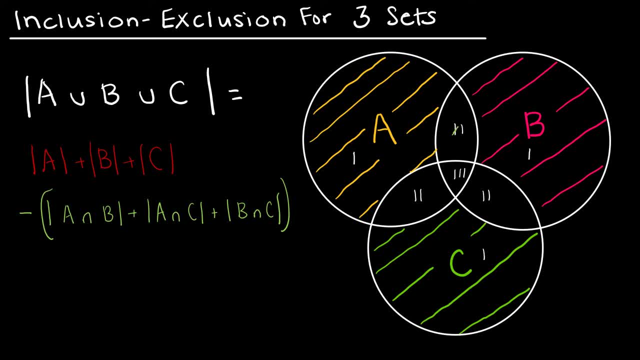 So I've taken away one of these, That's A intersect, That's A intersect B and one of these. And if I take away A intersect C, that's one of these and one of these. And if I take away B- intersect C, then that's one of these and, uh-oh, one of these. 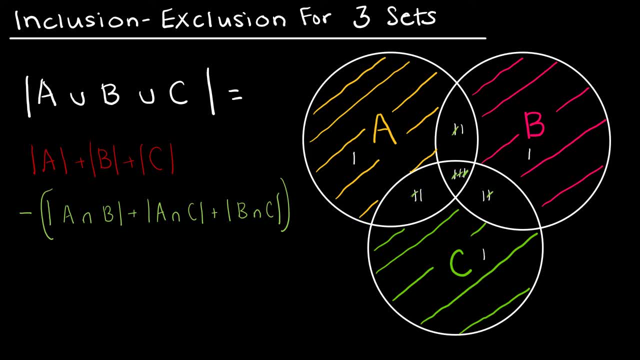 So where do I stand now? The yellow section's good, the pink section's good, the green section's good, And I'm just going to color these in in blue. These are okay now, because they're only being counted once instead of twice. 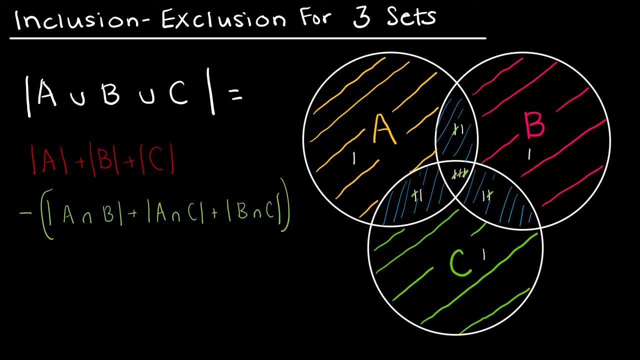 But now what's happened to the middle? It was counted three times. Now, all of the sudden, it's counted zero times, and that's not okay. So now I have to add back the number of elements in the intersection of A, B, C. 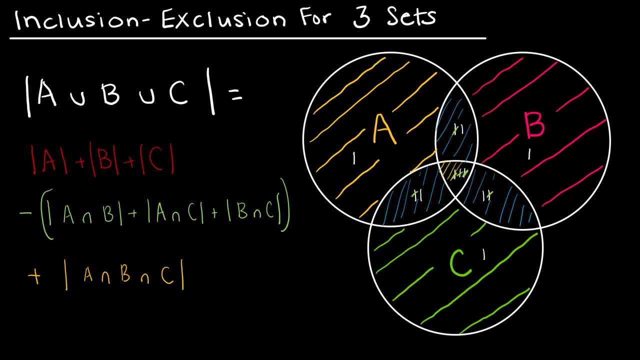 And that is just this region right here, And it has now only been counted one time. So this is how we would do this for three sets. So could I continue that for four sets? What pattern are we looking at? So it appears that we're going to add all of the elements that have of just one set. 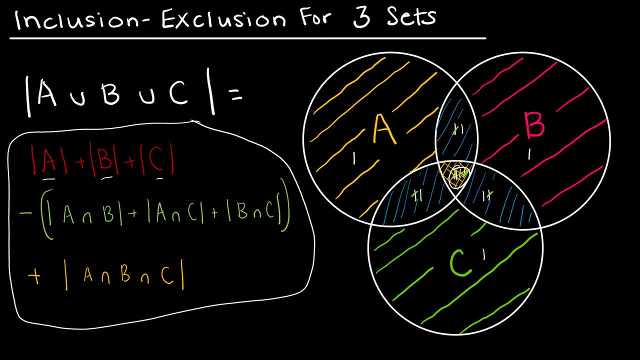 of each of these, each of the individual sets, then we're going to subtract the intersection of two sets, we're going to add the intersection of three sets. I guess if there were four sets then I would subtract the intersection of the four sets, etc. etc. etc. Let's take a look at an example now of a three set question. 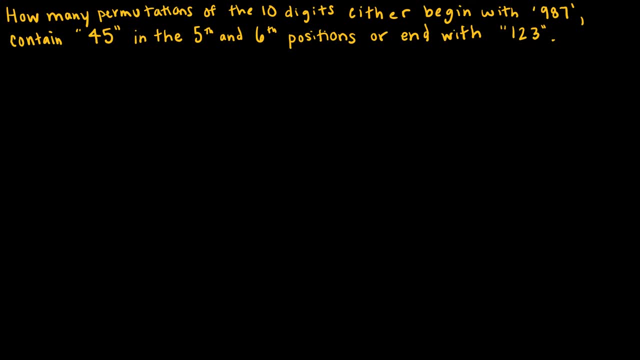 So how many permutations of ten digits? again the ten digits 0 through 9, either begin with 9,, 8, 7, contain 4,, 5 in the fifth and sixth positions, or end with 1,, 2, 3.. So again we're dealing with three different sets. We're going to call set A 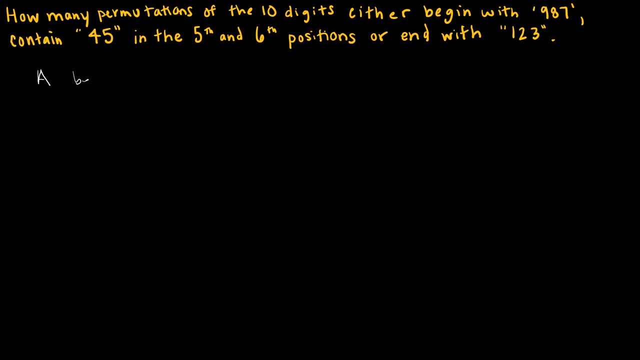 is going to be that it begins with 9,, 8,, 7.. Set B is that it contains 4,, 5, and 6 in the fifth and sixth position, and then set C is going to be that it ends in 1,, 2,, 3.. So we know, based on the formula we just talked about, if I need 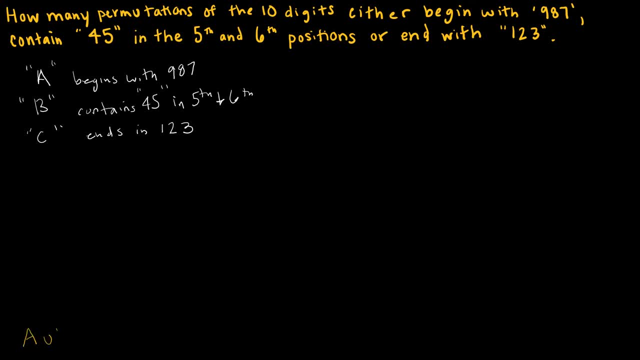 to find A union B union C, which is what I'm trying to find, then I'm going to take A plus B plus C. I'm adding all of the ones of size 1, I'm subtracting all of the intersection A intersect B. A, oops, A intersect C and B intersect C, and I'm adding A intersect B. 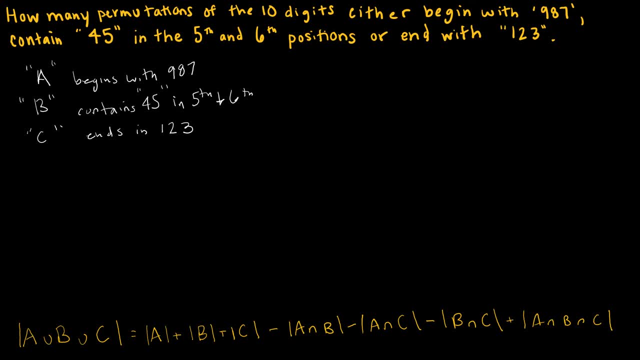 intersect C. Now again, think about it another way. you could have minus and then be finding the sum here, which we all know is the exact same thing. So whichever way makes the most sense to you is totally fine. I'm going to leave it written like this. So let's start to develop. 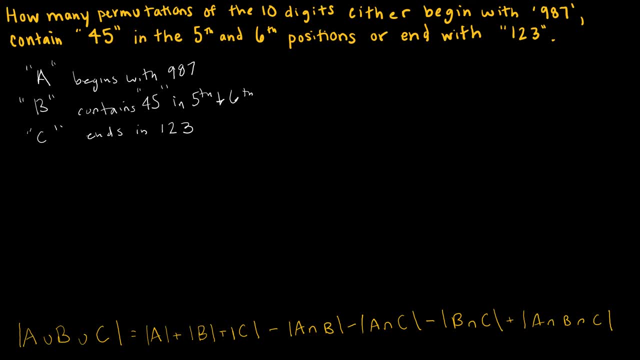 what values we'll be adding and subtracting in this question. So I'm going to look at 10, I'm just going to use this for all of them because I'm lazy- 1, 2,, 3,, 4,, 5,, 6,, 7,. 8,, 9,, 10,, 11,, 12,, 12,, 13,, 14,, 15,, 16,, 17,, 18,, 19,, 20,, 21,, 22,, 23,, 23,, 24,, 24,, 25,, 26,, 27,, 26,, 27,. 28,, 29,, 30,, 31,, 32,, 33,, 34,, 35,, 36,, 37,, 38,, 39,, 40,, 41,, 42,, 43,, 44,, 45,, 46,, 47,, 48,, 49,. 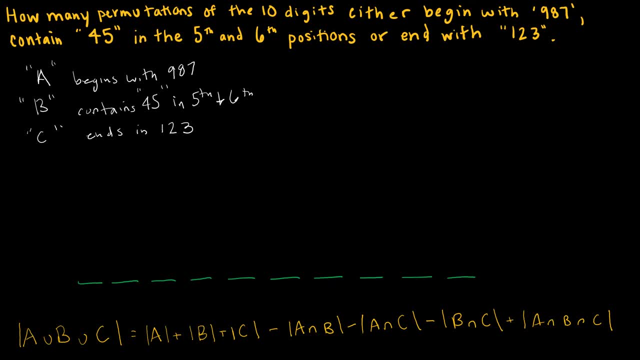 50,, 51,, 52,, 53,, 54,, 55,, 56,, 57,, 58,, 59,, 50.. So if I'm starting with A, if A begins with 9,, 8,, 7,, that leaves me with the values of. 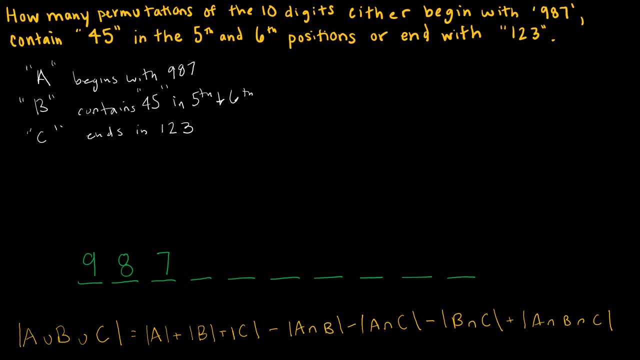 6,, 5,, 4,, 3,, 2,, 1, and 0, or 7 total values and 7 positions for me to permutate, which is 7 factorial, And then I'm going to write a value that's equal to 1.. 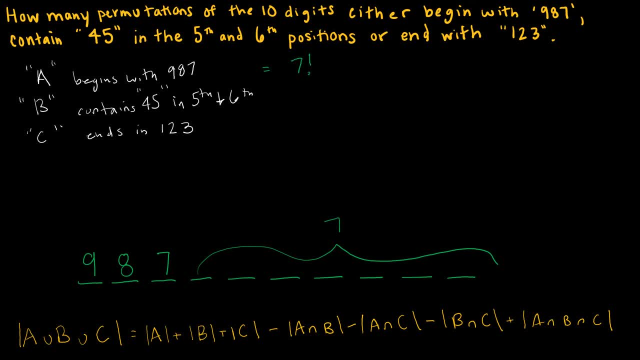 So I'm going to write a value that's equal to 1.. So if I'm starting with A, if A begins with 9,, 8,, 7,, that leaves me with values of 6, 5, And if it contains 4, 5 in the 5th and 6th position, so 1, 2, 3, 4,- this is the 5th position and this is the 6th position- that still leaves me with 1,, 2, 3,, 4,, 5,, 6,, 7,, 8 values to permutate in 8 positions, so that's 8 factorial. 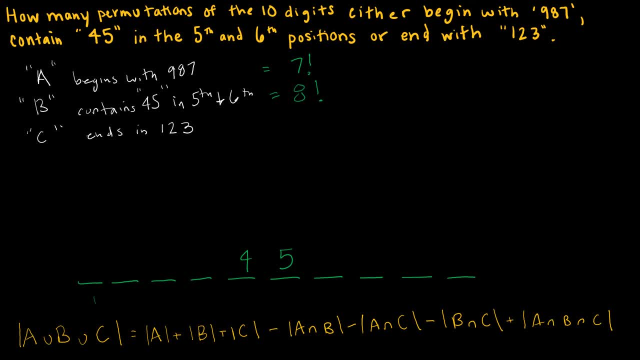 And then C. that ends with 1, 2, 3, again leaves me with these 7 to permutate. So that's all of the ones for the single set. so that's going to be here: 7 factorial plus 8 factorial plus 7 factorial. and now I need to look at the intersection. 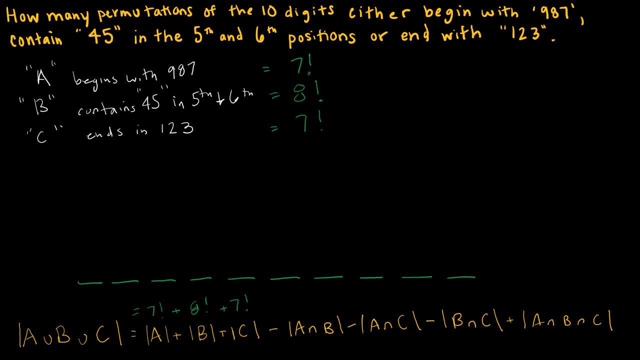 So A intersect B. A intersect B would be that it begins with 9,, 8, 7 and contains 4, 5 in the 5th and 6th position, which still leaves me with 1, 2,, 3,, 4, 5 to permutate. 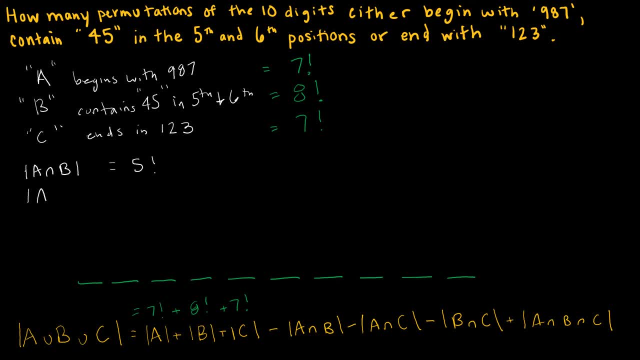 Now let's take a look at A intersect C. A intersect C would begin with 9,, 8, 7 and end in 1,, 2, 3, which leaves me with 1,, 2,, 3, 4 to permutate. 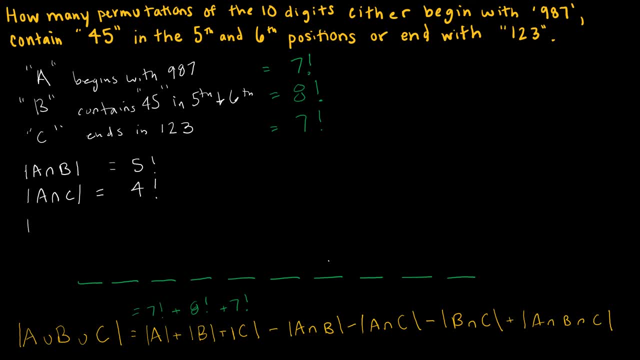 And then the last intersection of 2 would be B, intersect C, which contains 4, 5 in the 5th and 6th position and ends in 1,, 2, 3.. So that leaves me with 1.. 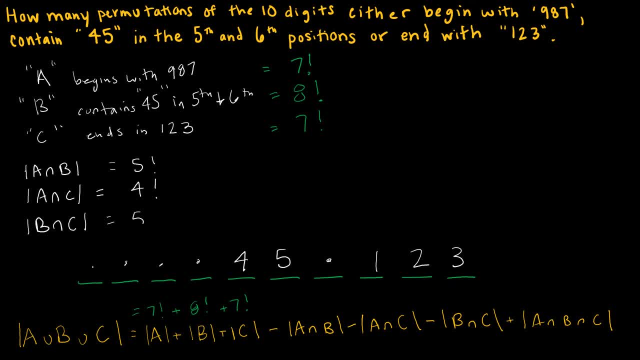 So that leaves me with 1,, 2,, 3,, 4,, 5,, 5 factorial. So I'm going to subtract 5, factorial, subtract 4, factorial, subtract 5, factorial. The very last one is A intersect B, intersect C, which I'm going to have to add back in, and that would be that it begins with 9,, 8,, 7.. 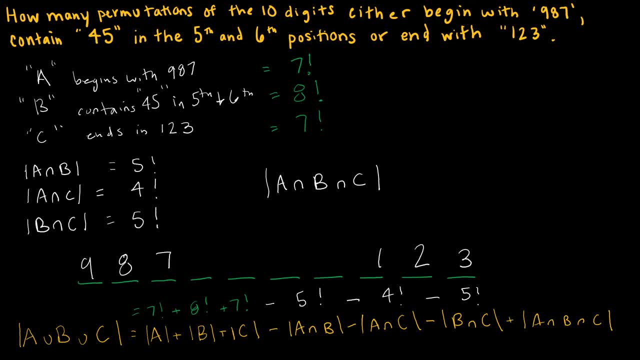 It ends in 1, 2.. So that leaves me with 1, 2, 3 and has 4 and 5 in the 5th and 6th position, which leaves me with 1, 2 values left to permutate. 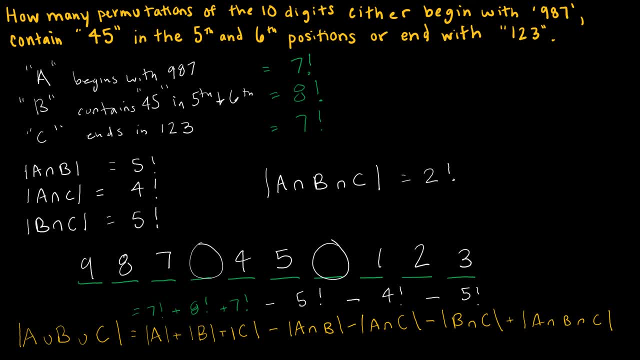 So that's 2 factorial, which is just 2. And that's all. Now, all I have to do is add and subtract using my calculator, And so what I end up with then is 50,138.. That's my calculator. 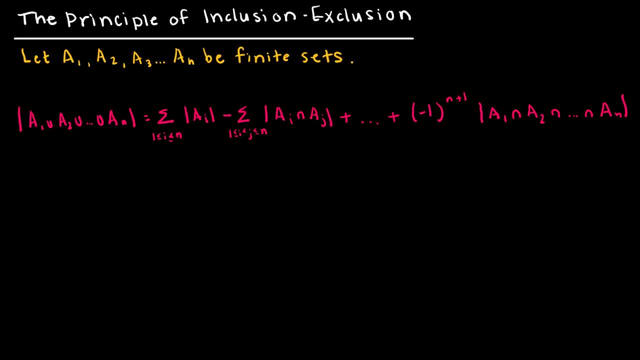 That's my final solution, So the generalization of the principle of inclusion-exclusion for any value of n. So we looked at a value of n equals 2 or 2 sets and the value of n equals 3 or 3 sets.